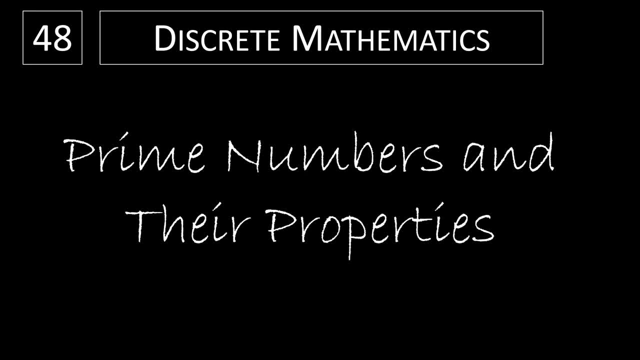 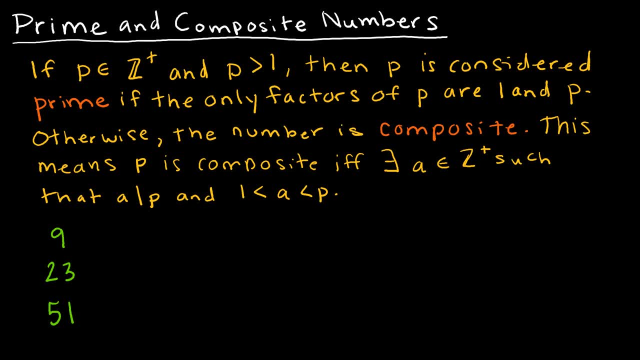 In this video we're going to take a look at prime numbers and their properties. You're likely already familiar with prime and composite numbers, but just in case you're not, let's go ahead and go through the definition. Notice: here we're talking strictly about. 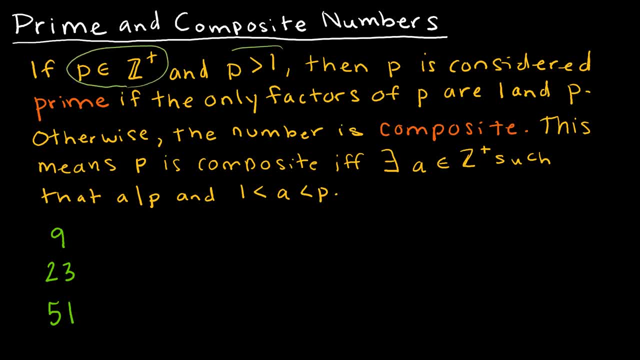 integers that are positive and that are greater than one. So the value of one is actually not considered prime or composite. so when we're starting this, we're really starting at the number two. So p is considered prime if the only factors of p are one and p. So if I try to break, 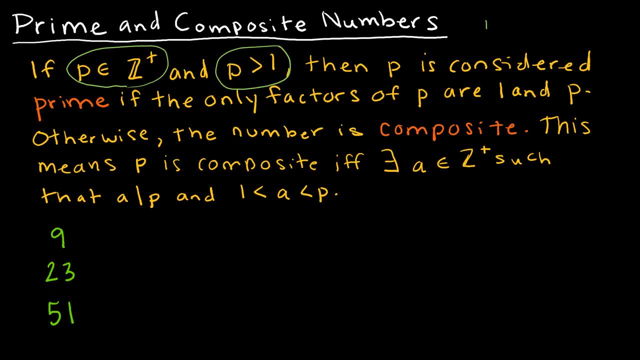 it down into factors. I'm only going to get one in itself. Otherwise, we consider the number composite, which means that there is some value a that divides p, and a has to be between one and p. So let's take a look at what we mean by that. First, let's talk about what some of the 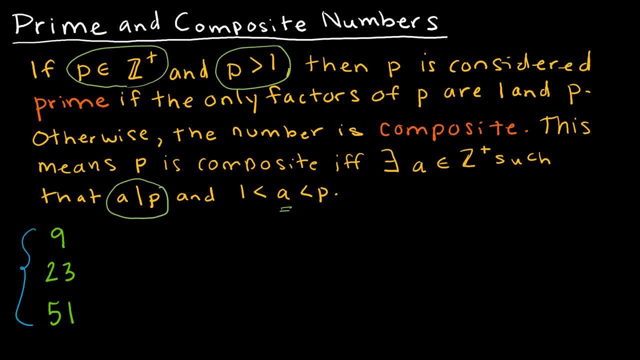 prime numbers are, and then we'll look at this example down here. So if I'm just looking at primes, one is not prime, but two is prime because the only numbers that go into two are one and two. Three is considered prime because, again, the only way to multiply to get three using integers. 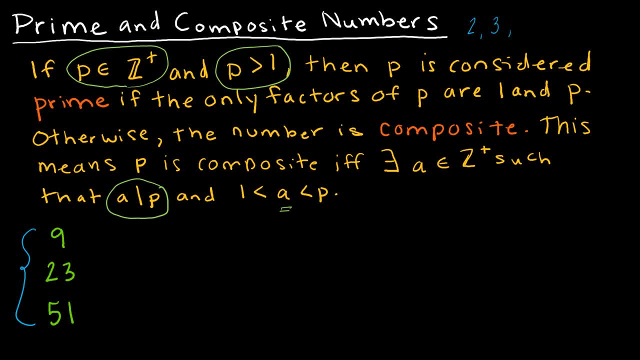 is one and three. Four would not be considered prime, because four can be written as one times four or two times two. Five is considered prime, six is not, and in fact from here on out every number that is even would not be prime, because two would go into. 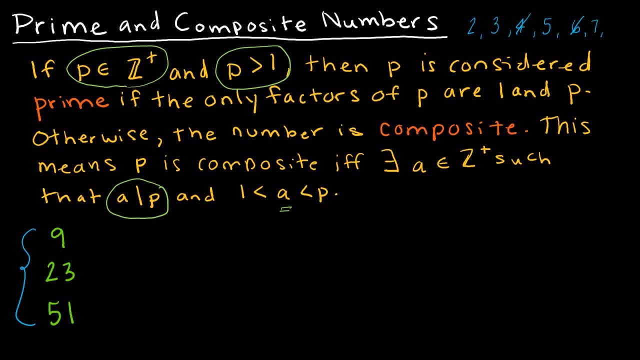 it. Seven is prime. I'm not even going to check eight. Nine is not prime because I can take three times three. So we get the idea and I'm not going to continue to make that list, but we understand exactly how to determine prime or not. So we'll start with nine and we've already sort of let 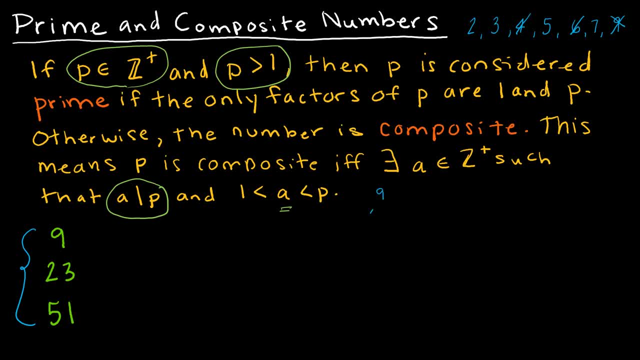 the cat out of the bag there, but I want to bring you back to probably middle school when you learn about factor trees. When we made a factor tree we said: let's make a tree where we find the factors of our value that are prime numbers. So I'm going to be looking at two and three and 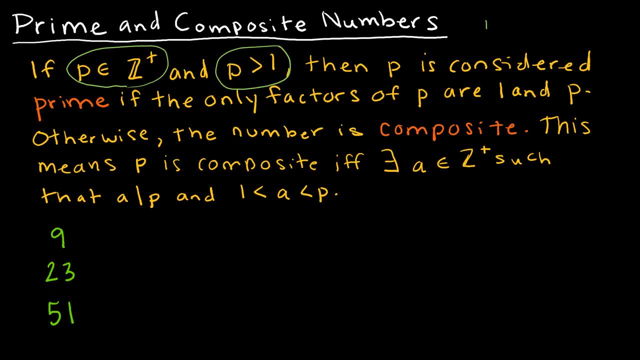 it down into factors. I'm only going to get one in itself. Otherwise, we consider the number composite, which means that there is some value a that divides p, and a has to be between one and p. So let's take a look at what we mean by that. First, let's talk about what some of the 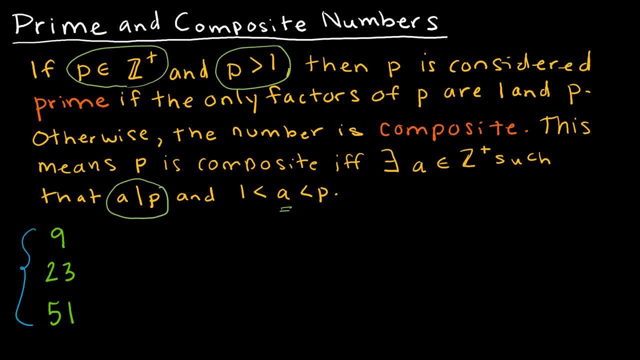 prime numbers are, and then we'll look at this example down here. So if I'm just looking at primes, one is not prime, but two is prime because the only numbers that go into two are one and two. Three is considered prime because, again, the only way to multiply to get three using integers. 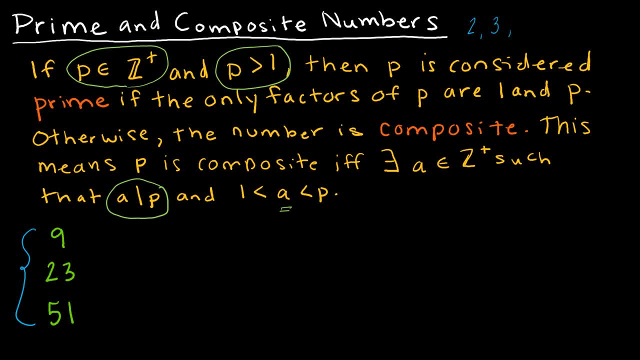 is one and three. Four would not be considered prime, because four can be written as one times four or two times two. Five is considered prime, six is not, and in fact from here on out every number that is even would not be prime, because two would go into. 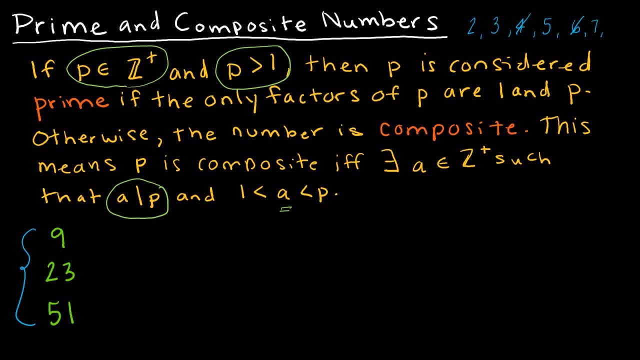 it. Seven is prime. I'm not even going to check eight. Nine is not prime because I can take three times three. So we get the idea and I'm not going to continue to make that list, but we understand exactly how to determine prime or not. So we'll start with nine and we've already sort of let 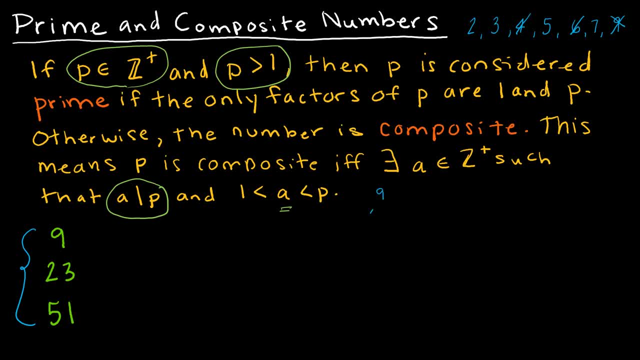 the cat out of the bag there, but I want to bring you back to probably middle school when you learn about factor trees. When we made a factor tree we said: let's make a tree where we find the factors of our value that are prime numbers. So I'm going to be looking at two and three and 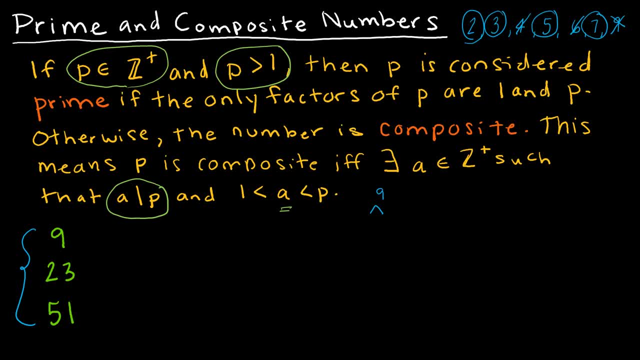 five and seven and all of the other primes that I know, and say what primes could I multiply to get nine? And in this case I can multiply three times three. So this is called my prime factorization. but notice what this says. That means 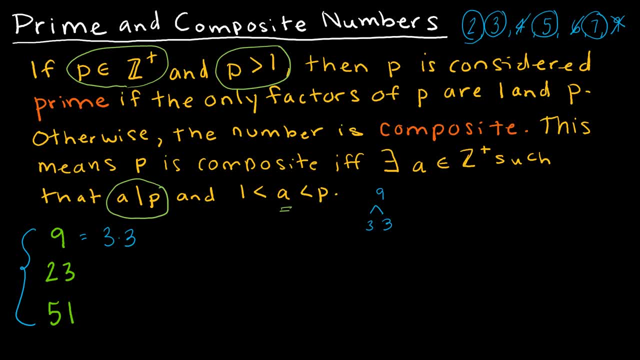 the number is composite, if there exists some a, such that a divides p, So obviously three divides nine, and therefore this is considered a composite number. So now let's take a look at the number 23. 23. Two doesn't go into it. Three doesn't go into it, Five doesn't go into it, Seven doesn't go. 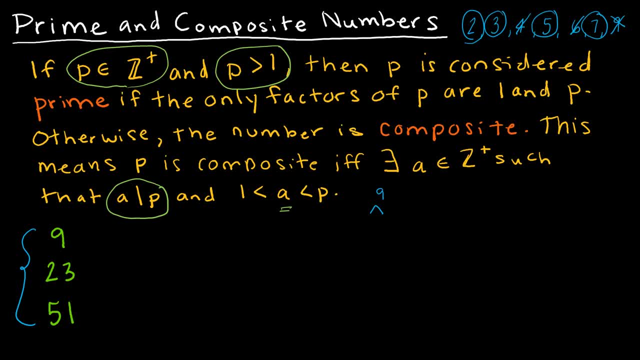 five and seven and all of the other primes that I know, and say what primes could I multiply to get nine? And in this case I can multiply three times three. So this is called my prime factorization. but notice what this says. That means 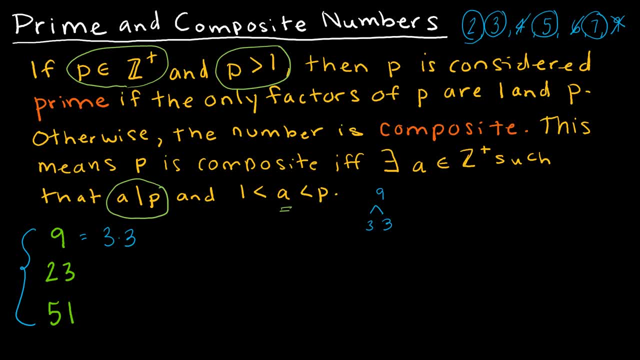 the number is composite, if there exists some a, such that a divides p, So obviously three divides nine, and therefore this is considered a composite number. So now let's take a look at the number 23. 23. Two doesn't go into it. Three doesn't go into it, Five doesn't. 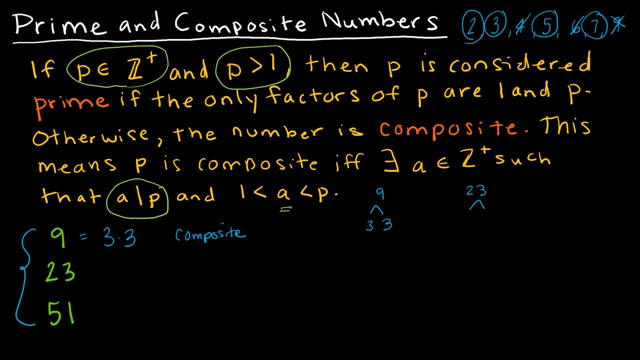 go into it. Seven doesn't go into it. The next prime number after that is 11.. That doesn't go into it. Thirteen doesn't go into it. Thirteen doesn't go into it. Thirteen doesn't go into it. 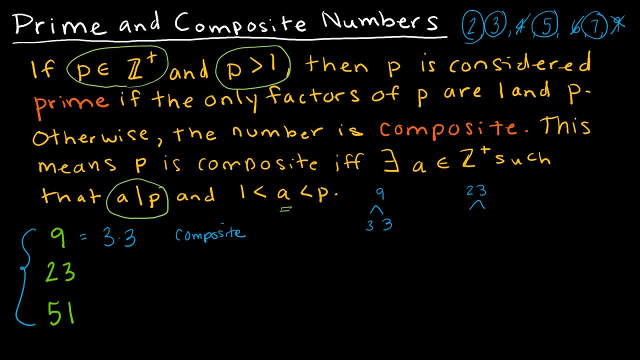 And I'm going to stop there. This one doesn't break down. This one can only be written as one times 23. And that is the definition of a prime number, is that it's only divisible by one in itself. Our last one is 51. And again we're going to talk a little bit more about when I can stop. 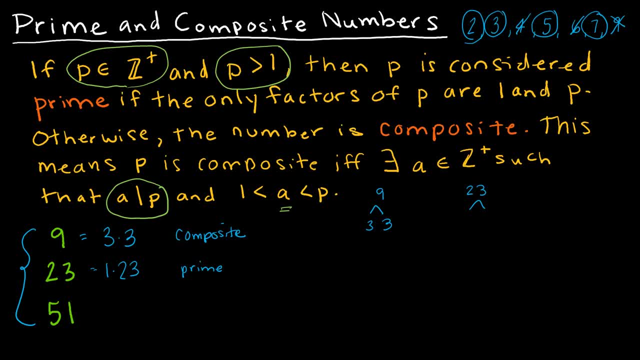 checking. Notice I stopped checking at 13.. We're going to talk more about that in a little bit, but for now just stick with me For 51,. a lot of people you know start looking at these larger numbers, not the 51s- all that large. 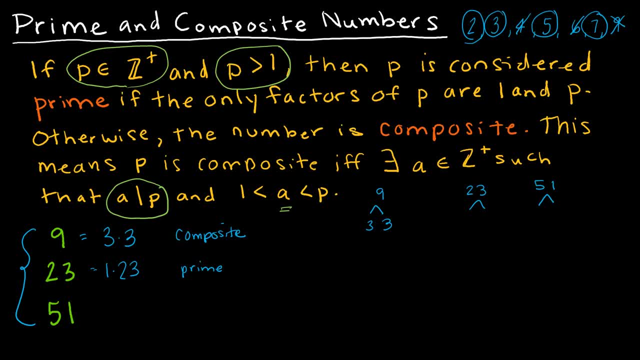 but a lot of people say: you know what I don't want to. we're just going to call it prime because it's too big and I don't want to go through all of the values. But if you'll remember, there are some divisibility rules And if you don't know, them off the top of your head, 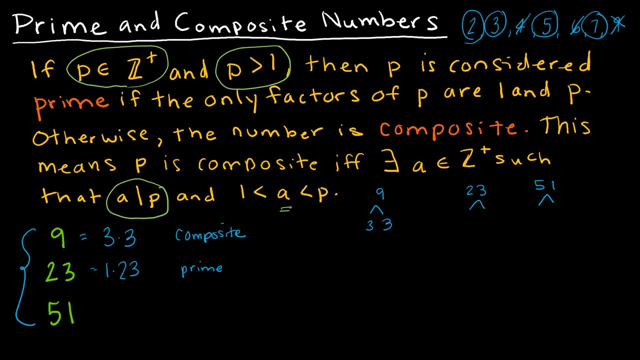 not a bad idea to Google those, But one of the easier ones is the number or the rule for three. The rule for three says if you take the digits of the number and the sum of those digits is divisible by three, then the number itself is divisible by three. 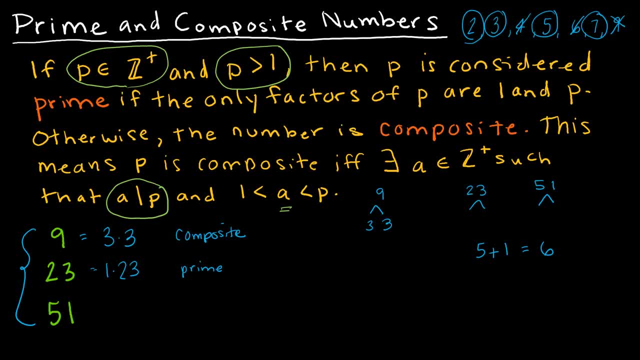 And notice: five plus one equals six, which is divisible by three. So that means if I were to break this down, it would be three times something, And in this case that is three times 17.. And again, because I can write this as a product of primes. 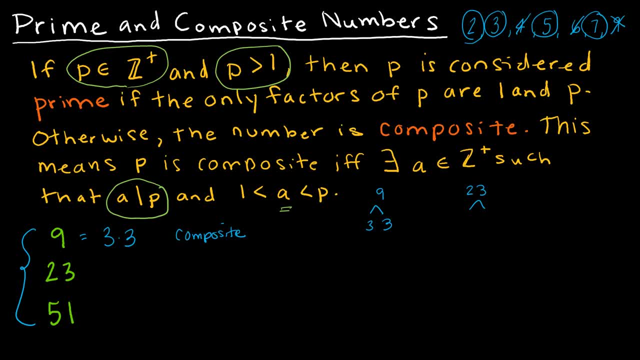 into it. The next prime number after that is 11.. That doesn't go into it. Thirteen doesn't go into it And I'm going to stop there. This one doesn't break down. This one can only be written as one times 23.. And that is the definition of a prime number, is that it's only divisible by one. 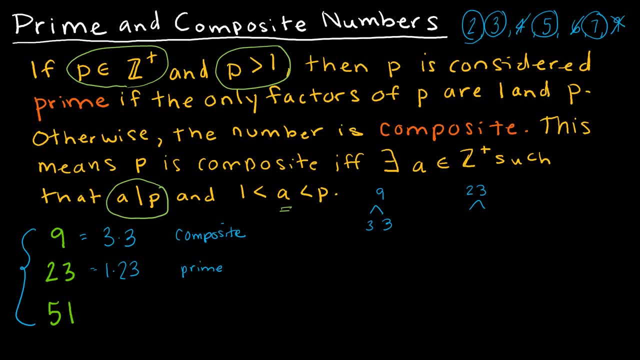 in itself. Our last one is 51. And again we're going to talk a little bit more about when I can stop checking. Notice I stopped checking at 13.. We're going to talk more about that in a little bit, But for now just stick with me For 51,. 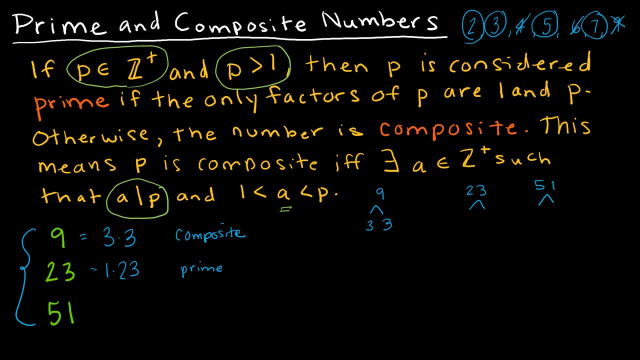 a lot of people, you know, start looking at these larger numbers, not the 51s, all that large. But a lot of people say: you know what I don't want to. we're just going to call it prime because it's too. 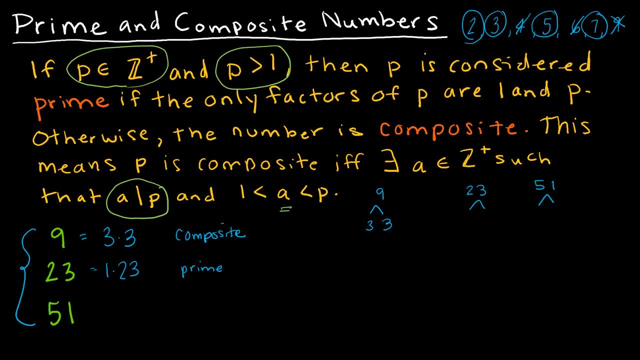 big And I don't want to go through all of the values, But, if you'll remember, there are some divisibility rules And if you don't know them off the top of your head, not a bad idea to Google those. But one of the easier ones is the number or the rule for three. The rule for three says: 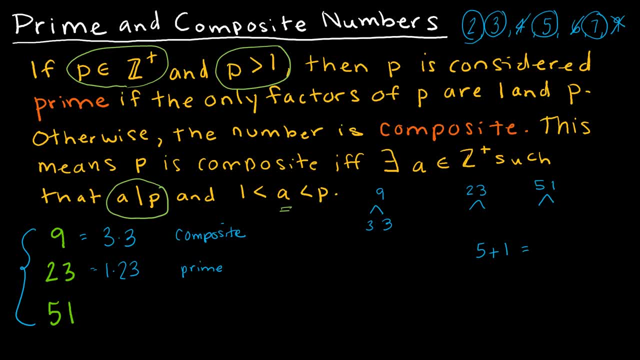 if you take the digits of the number and the sum of those digits is divisible by three, then the number itself is divisible by three. And notice: five plus one equals six, which is divisible by three. So that means if I were to break this down, it would be three times something, And in this case that is three times 17.. And 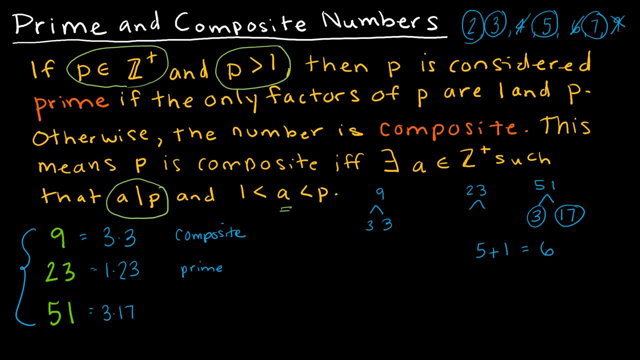 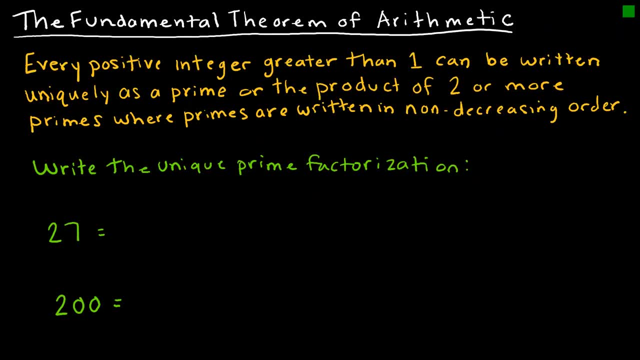 again, because I can write this as a product of primes, not just one in itself. this is considered a composite number, So we really just touched on this a moment ago. But the fundamental theorem of arithmetic says every positive integer greater than one can be written. 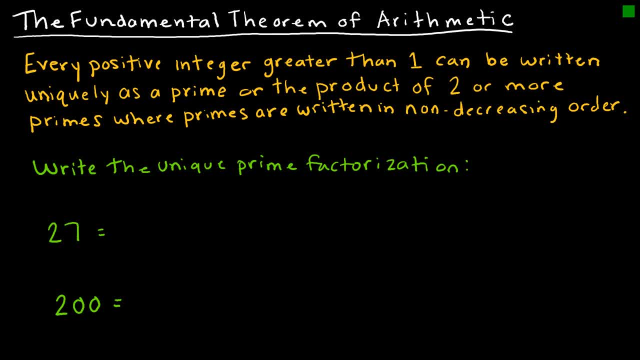 uniquely as a prime. So when we looked at the number 23,, that was a prime or the product of two or more primes, where primes are written in non decreasing order. So again, all this is saying is look at the factor tree or create the factor tree. Typically, we just do this in our head. 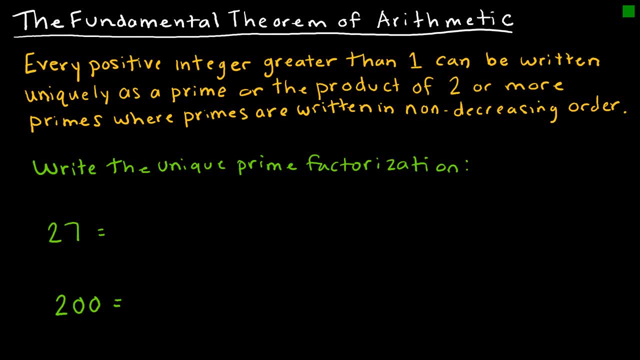 you know, because we're not in sixth grade anymore. So, looking at the prime factorization, I would say 27 is not divisible by two, but it's divisible by three. And that leaves me with 27 divided by three, which is nine. that I would say well, three goes into. 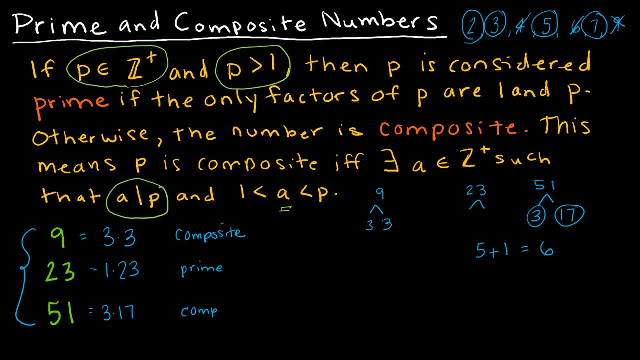 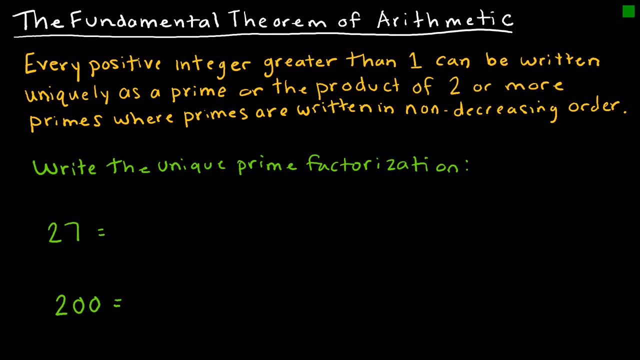 not just one in itself. this is considered a composite number. So we really just touched on this a moment ago. the fundamental theorem of arithmetic says every positive integer greater than one can be written uniquely as a prime. So when we looked at the number 23, that was a prime or the product of. 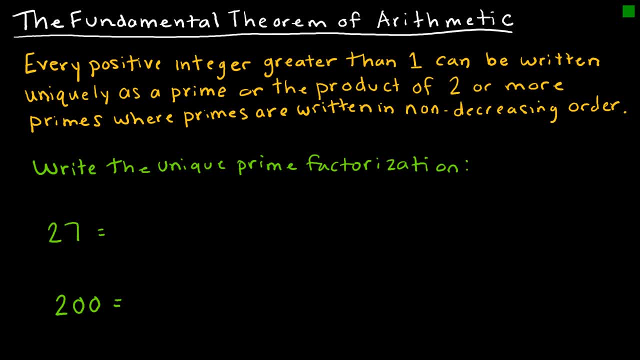 two or more primes, where primes are written in non decreasing order. So again, all this is saying is: look at the factor tree or create the factor tree. Typically, we just do this in our head because we're not in sixth grade anymore. So, looking at the 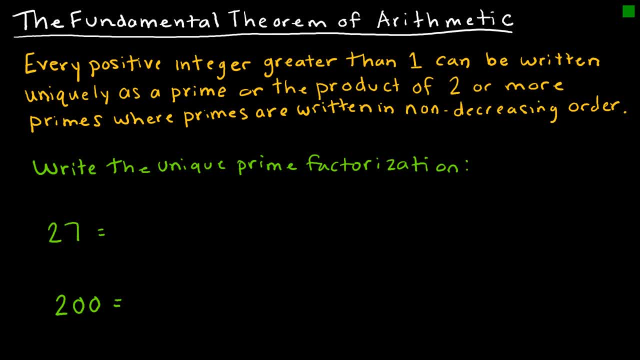 prime factorization I would say: 27 is not divisible by two, but it's divisible by three. And that leaves me with 27 divided by three, which is nine. that I would say: well, three goes into nine. And if I take nine divided by three, I get three. And so this is three times three times three. 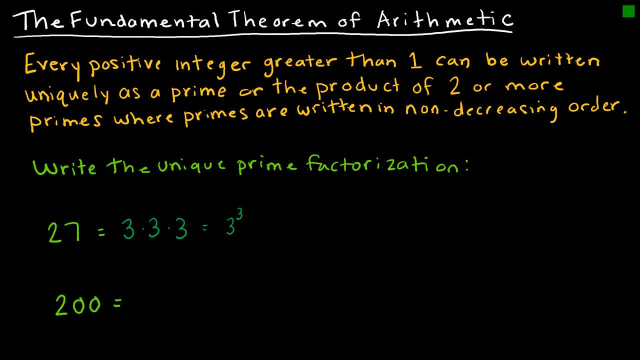 which of course we could write as three to the third. we can do the same thing with 200.. Typically we start with the lowest ones because again, we're non decreasing order. So I would say: does to go into 200? It does. it leaves me with 100.. Does to go into 100?? Yes, it does, It leaves. 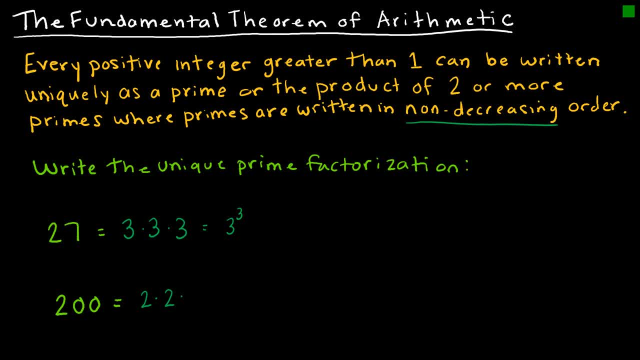 me with 50.. Does to go into 50?? Yes, it does. It leaves me with 25.. And then two no longer goes into 25.. And three does not go into 25.. But five does go into 25, leaving me with a remainder of five. 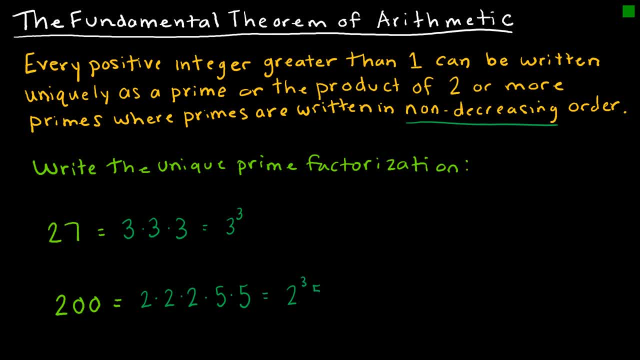 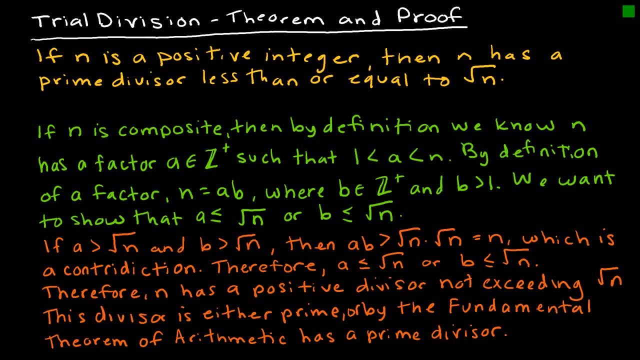 And so my prime factorization would be two to the third, five squared. So previously we looked at whether or not 23 was prime And I sort of alluded to: hey, wouldn't it be nice if we knew how many numbers we had to check to determine if it was prime. 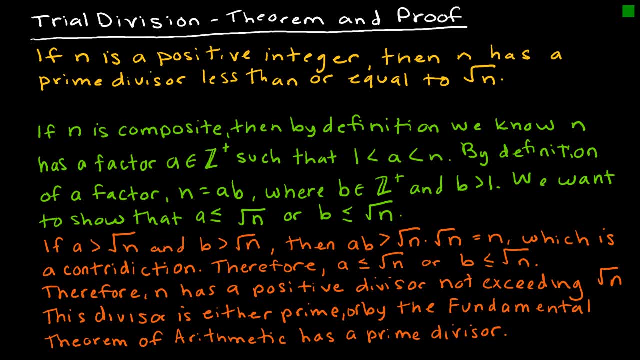 And that is what this theorem is going to help us move towards. So this is not a great theorem. necessarily it does, I guess, cut the playing field in half, But it's not the best way, I guess, to determine if a number is prime. So here's our theorem: If n is a positive, 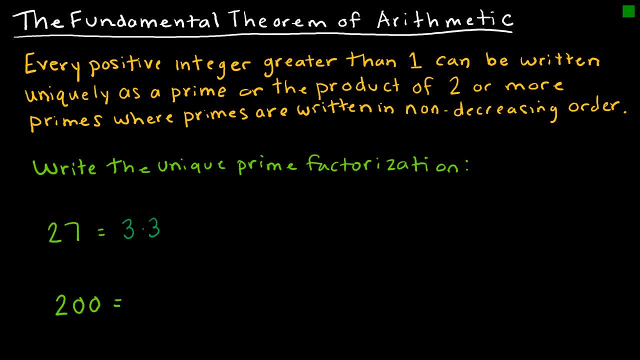 nine, And if I take nine divided by three, I get three, And so this is three times three times three, which of course we could write as three to the third. We can do the same thing with 200.. Typically we start with the lowest ones because, again, we're non decreasing order. 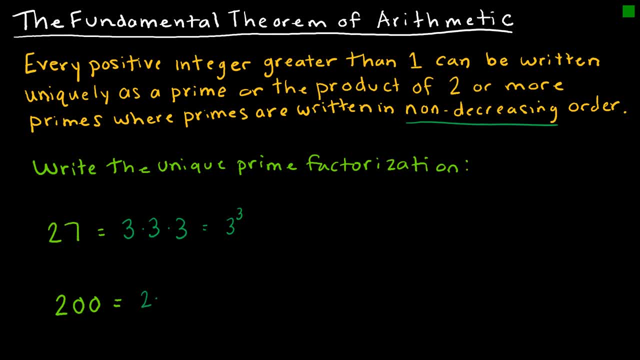 So I would say: does two go into 200? It does. it leaves me with 100.. Does two go into 100? Yes, it does. It leaves me with 50.. Does two go into 50? Yes, it does. It leaves me with 25.. 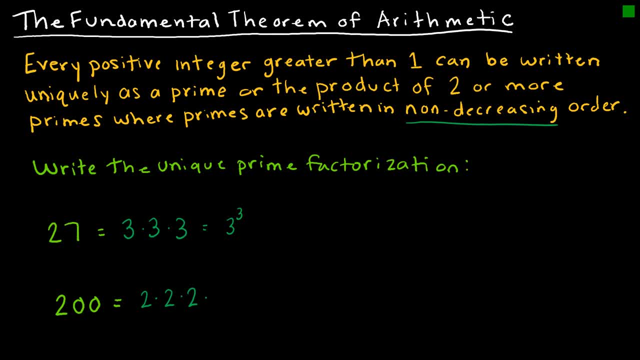 And then two no longer goes into 25.. And three does not go into 25.. But five does go into 25, leaving me with a remainder of five, And so my prime factorization would be two to the third, five squared. 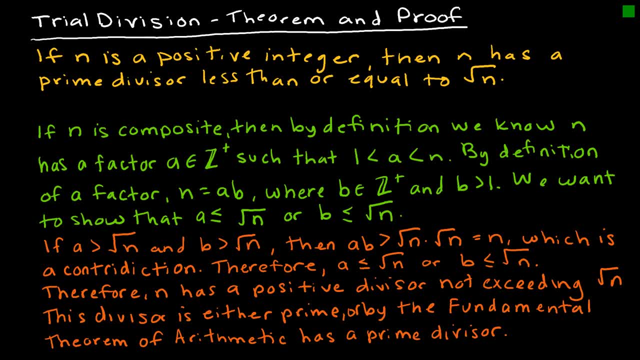 So previously we looked at whether or not 23 was prime And I sort of alluded to: hey, wouldn't it be nice if we knew how many numbers we had to check to determine if it was prime? And that is what this theorem is going to help us move towards. So this is not a great theorem. 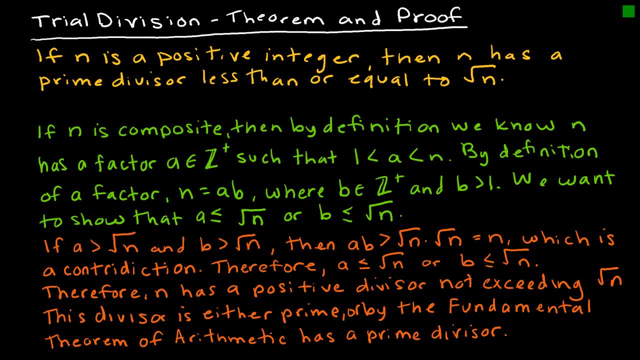 necessarily. It does, I guess, cut the playing field in half, But it's not the best way, I guess, to determine if a number is prime. So here's our theorem: If n is a positive integer, then n has a prime divisor less than or equal to radical n. So I want to talk about 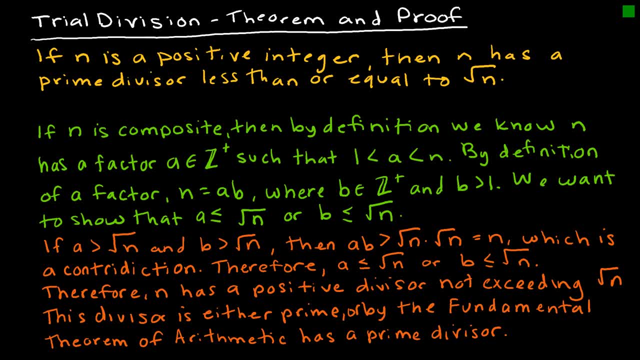 the proof of that, because I promised to include more proofs And so in green I have laid out for you essentially how we're going to prove it. So we start by saying: if n is composite, then by definition we know that n has a factor a, that is a positive integer, such that one is. 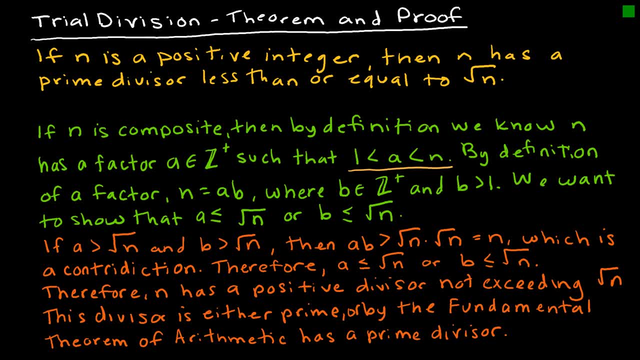 less than a is less than n. So this is just the definition of a composite number that we talked about a few moments ago. And why did I assume that n is composite? Because obviously, if it was prime, it's not going to have a divisor. So, by definition of a factor, because we're saying a is a factor, 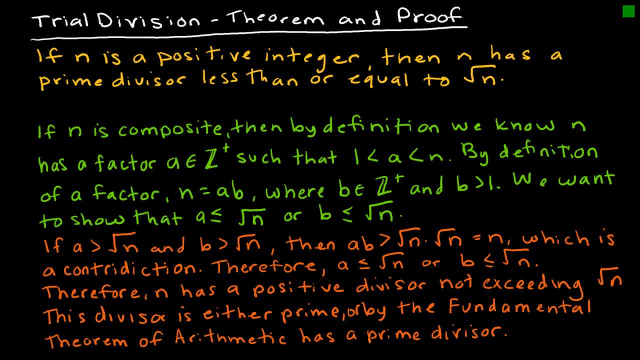 integer, then n has a prime divisor less than or equal to radical n. So I want to talk about the proof of that, because I promised to include more proofs And so in green I have laid out for you essentially how we're going to prove it. So we start by saying: if n is composite, 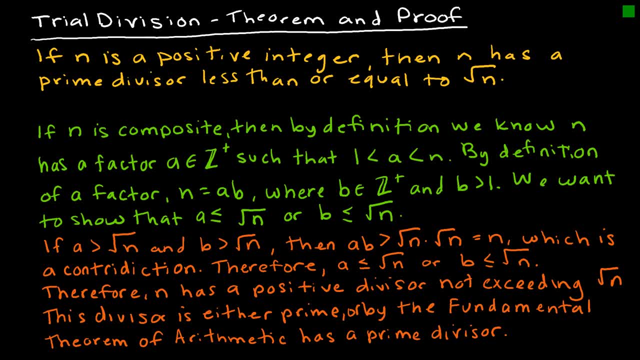 then by definition we know that n has a factor a, that is a positive integer, such that one is less than a is less than n. So this is just the definition of a composite number that we talked about a few moments ago. And why did I assume that n is composite? Because obviously, if it was prime, 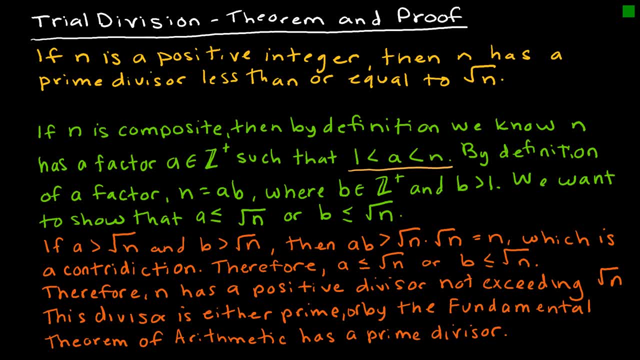 it's not going to have a divisor. Okay, So by definition of a factor, because we're saying a is a factor, that just means that n is a composite. So if n is a composite, then n is a composite. I can write n as a times some other number and I've chosen b, where b is also a positive. 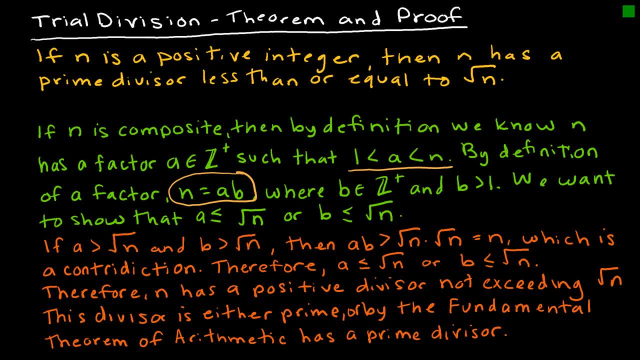 integer greater than one. And what I'm trying to do, what I want to show is that a is less than or equal to radical n, or b is less than or equal to radical n. So why do I want to show that? Because it says n has a prime divisor less than or equal to radical n. And so if I show that a is 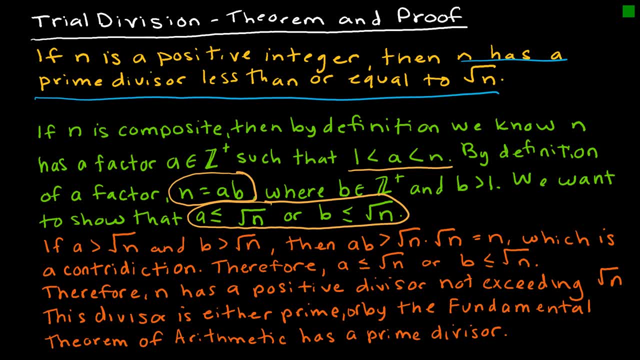 less than or equal to radical n, or b is less than or equal to radical n, then I'm trying to show that a is less than or equal to radical n, then I have proved that theorem. So here's the proof. If a is: 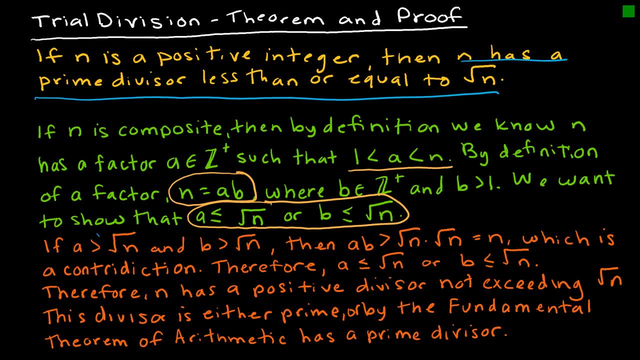 greater than radical n and b is greater than radical n. So notice, here I've assumed that they're greater, to see what would happen if that were true. then a, b is greater than radical n times radical n, which is of course n, which is a contradiction because it cannot be greater than n. 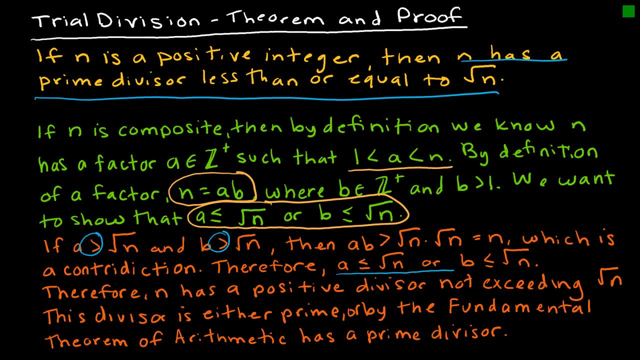 Therefore, either a is less than radical n or b is less than or equal to radical n. So why did that help me? Because then n has a positive divisor not exceeding radical n, which is either a or b. we don't have to specify which The divisor is, either prime. 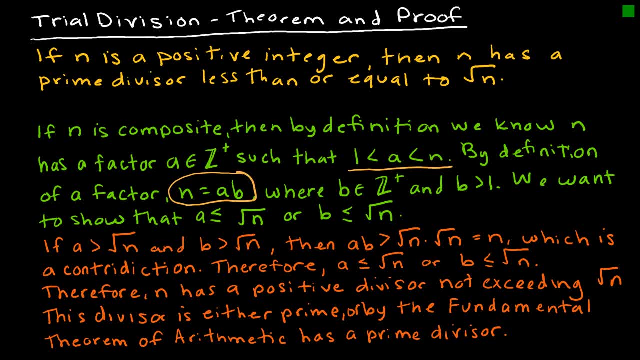 then this is a positive integer, So we can write n as a times some other number, and I've chosen b, where b is also a positive integer greater than one, And what I'm trying to do, what I want to show is that a is less than or equal to radical n, or b is less than or equal to radical n. So 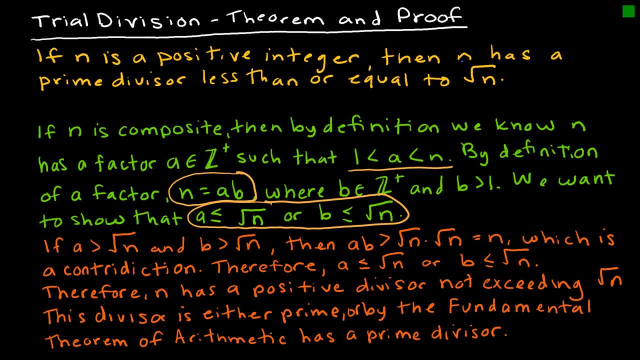 why do I want to show that? Because it says n has a prime divisor less than or equal to radical n. And so if I show that a is less than or equal to radical n or b is less than or equal to radical n, then I'm going to be able to show that a is less than or equal to radical n, And so I'm going to. 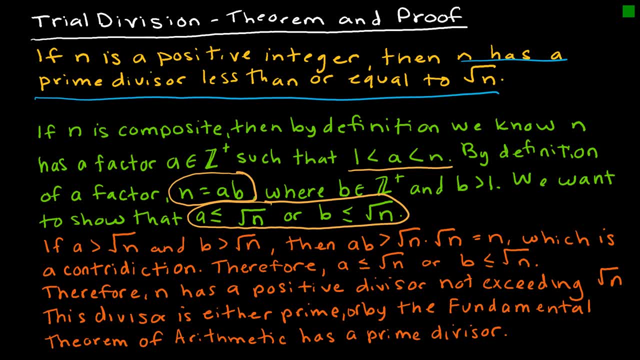 show that a is less than or equal to radical n, then I have proved that theorem. So here's the proof: if a is greater than radical n and b is greater than radical n- So notice, here I've assumed that they're greater, to see what would happen if that were true- then a- b is greater. 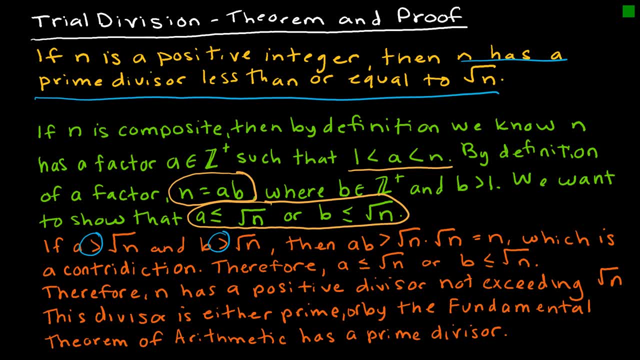 than radical n times radical n, which is, of course, n, which is a contradiction because it cannot be greater than n. Therefore, either a is less than radical n or b is less than or equal to radical n. So why did that help me? Because then n has a positive divisor not exceeding radical n, which is: 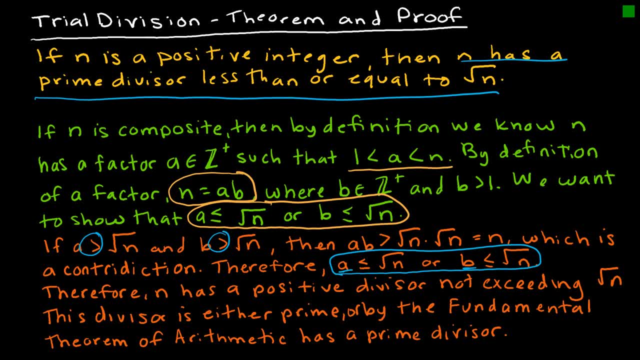 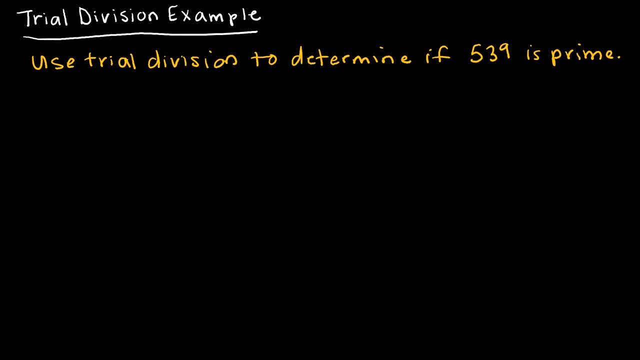 either a or b. we don't have to specify which The divisor is, either prime or by. the fundamental theorem of arithmetic has a prime divisor. Therefore, we have proved the theorem. Now that we have proved the theorem, let's go ahead and use it to determine if 539 is less than or equal to radical n. 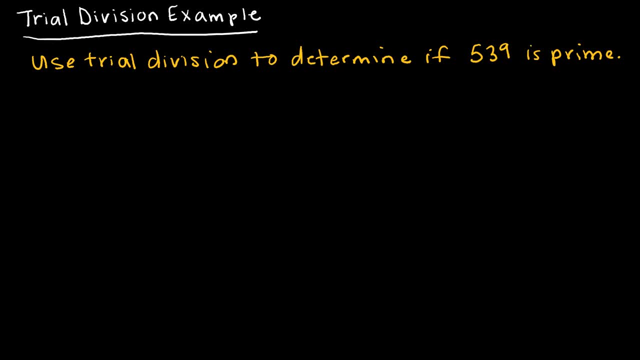 And we just need to find that the przez of the prata we've defined as 539 is prime. So recall what our theorem told us is that, instead of having to check all of the primes up to 539, we just have to find 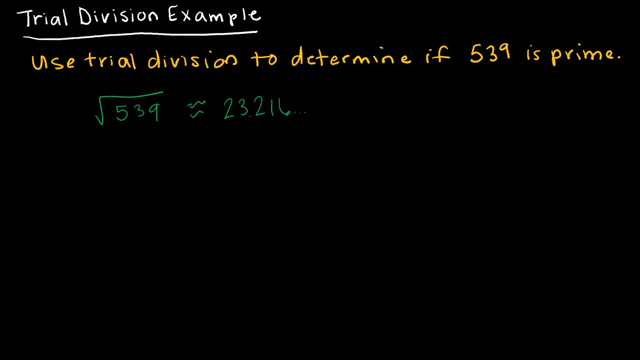 what is radical 539.. And radical 539 is about 23.216, and it continues on. Trial division says I have to check all of the primes that are less than 23.216. I have to check all of the primes that are less than 23.216. 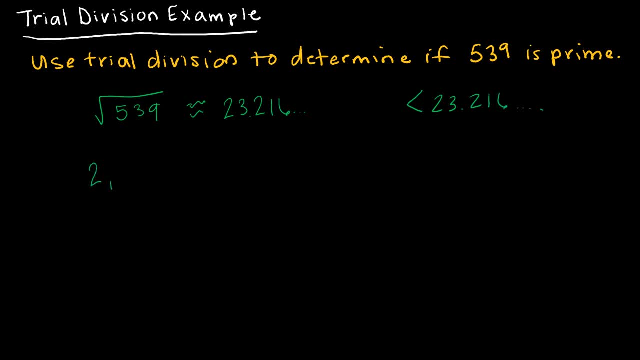 Which means I have to check 2, and 3, and 5, and 7, and 11, and 13, and 17, and 19, and 23.. Because 23 is less than 23.216.. 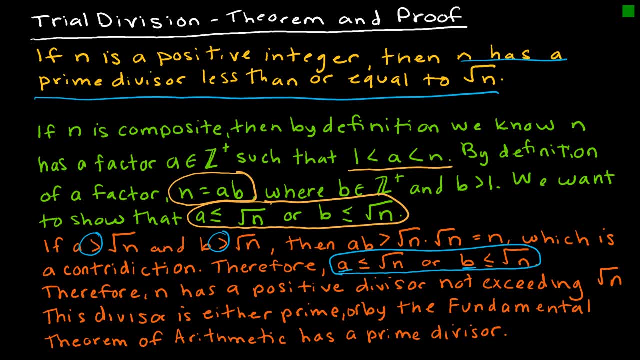 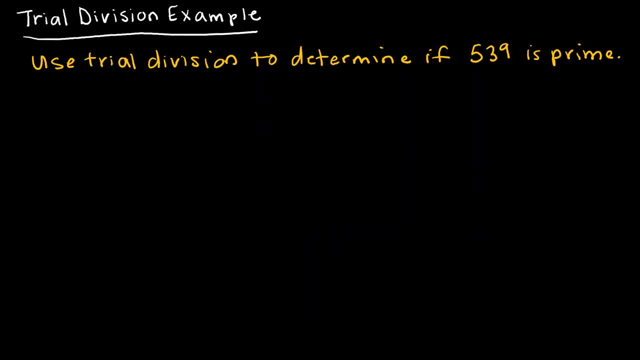 or by the fundamental theorem of arithmetic, has a prime divisor. Therefore, we have proved the theorem. Now that we have proved the theorem, let's go ahead and use it to determine if 539 is prime. So recall what our theorem told us is that, instead of having to check all of the primes, 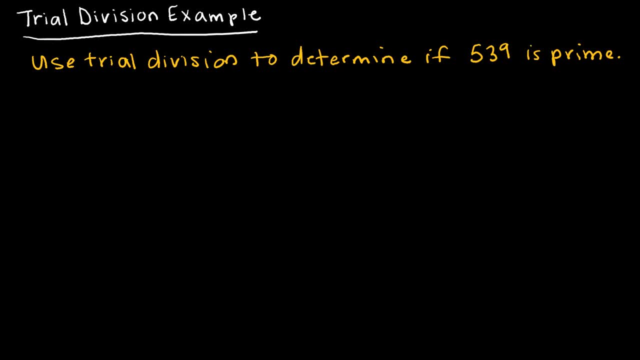 up to 539,. we just have to find what is radical 539.. And radical 539 is about 23.216, and it continues on. Trial division says I have to check all of the primes that are less than 23.216,. 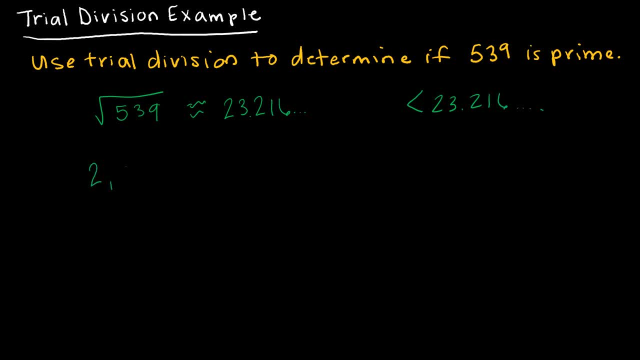 Which means I have to check 2, and 3, and 5, and 7, and 11, and 13, and 17, and 19, and 23.. Because 23 is less than 23.216.. 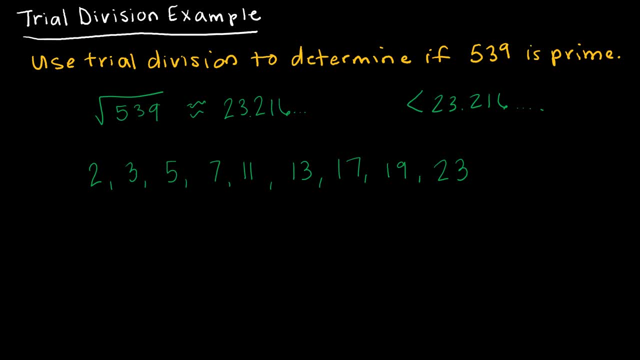 So, honestly, what I would do is I would start with 2 and say: okay, does 2 go into 539?? No, because 539 is obviously an odd number. Does 3 go into 539?? Well, again I can check: 5 plus 3 plus 9, which is 8, plus 9,, which is 17.. 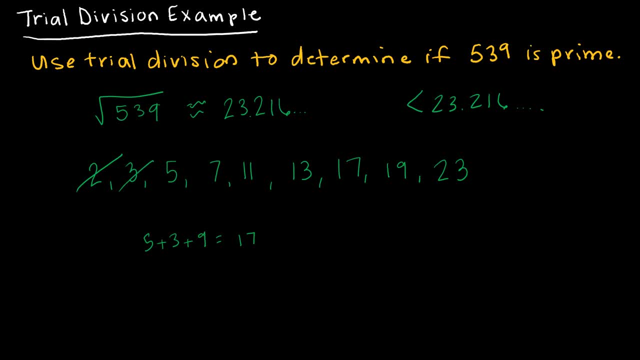 And 3 doesn't go into 17,. so 3 doesn't go into 539.. Obviously, 5 doesn't go into 539 because the divisibility rule is that it would end in a 5 or a 0.. So now let's check 7.. And again, you can just do this with your calculator. 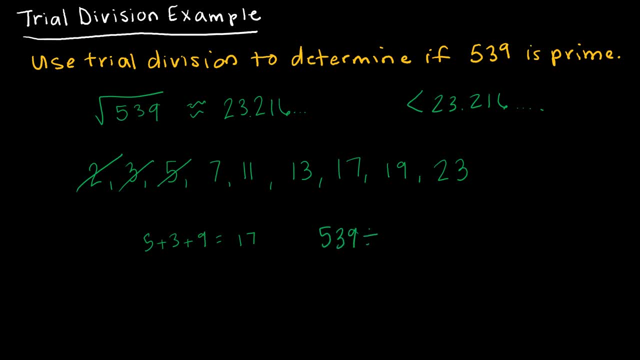 And when I did 539 divided by 7, I get 77.. And because I have found a value that goes into 539- beyond just 1 and 539, this is considered a composite number. Deceive of Eratosthenes. 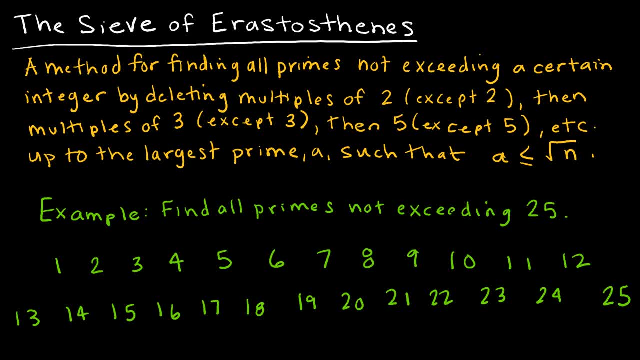 Deceive of Eratosthenes is essentially another way for us to find all primes that don't exceed a certain integer. And what we're going to do is we're going to delete multiples of 2, because 2 is obviously a prime number, except for the number 2.. 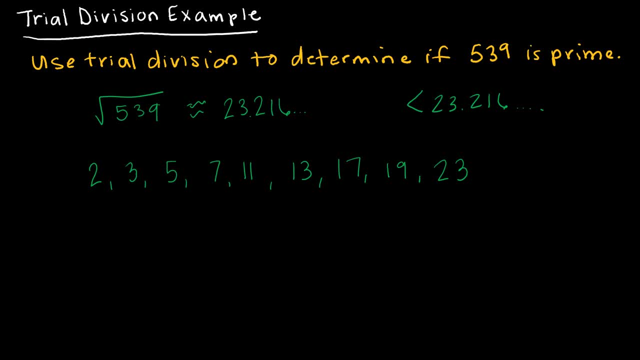 So, honestly, what I would do is I would start with 2 and say: okay, does 2 go into 539?? No, because 539 is obviously an odd number. Does 3 go into 539?? Well, again I can check: 5 plus 3 plus 9, which is 8, plus 9,, which is 17.. 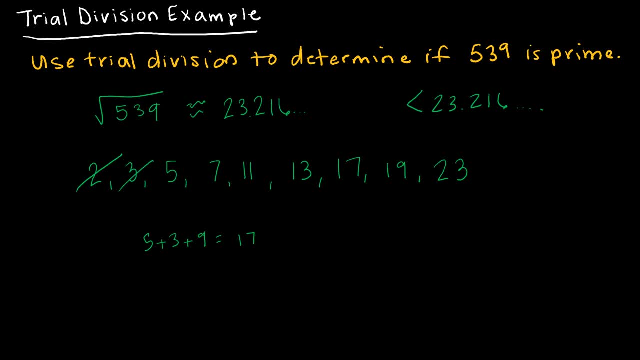 And 3 doesn't go into 17,. so 3 doesn't go into 539.. Obviously, 5 doesn't go into 539, because the divisibility rule is that it would end in 539.. It would end in a 5 or a 0.. 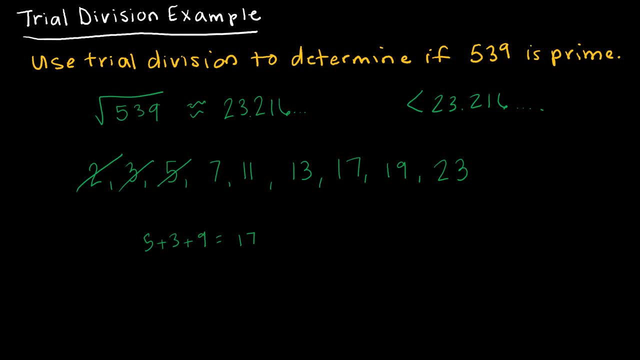 So now let's check 7.. And again, you can just do this with your calculator, And when I did 539 divided by 7, I get 77.. And because I have found a value that goes into 539, beyond just 1 and 539,. 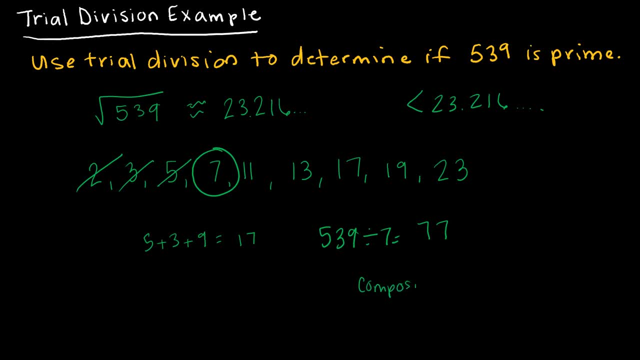 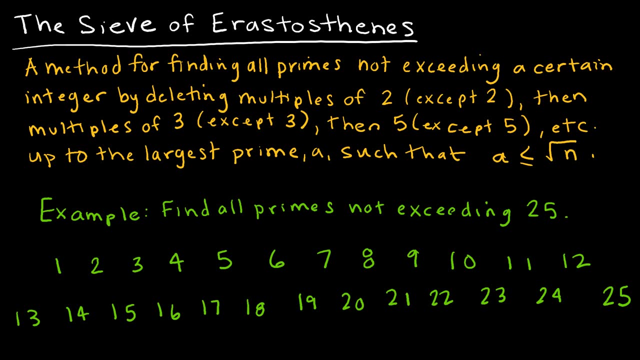 this is considered a composite number. Deceive of Eratosthenes. Deceive of Eratosthenes is essentially another way for us to find all primes that don't exceed a certain integer, And what we're going to do is we're going to delete multiples of 2,. 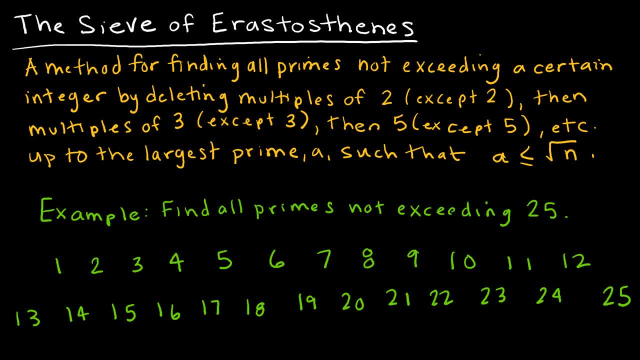 because 2 is obviously a prime number, except for the number 2.. Then we're going to delete multiples of 3, because 3 is obviously a prime number, but we're not going to delete 3.. And then 5, etc. through all of the largest primes, such that a is less than or equal to n. 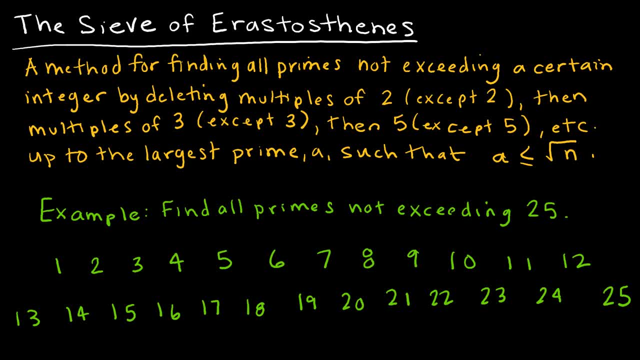 Sorry. a is less than or equal to the square root of n, So I've given us a sort of a simple example. I'm using 25.. So I would take square root of 25.. So a is less than or equal to the square root of 25, which is 5.. 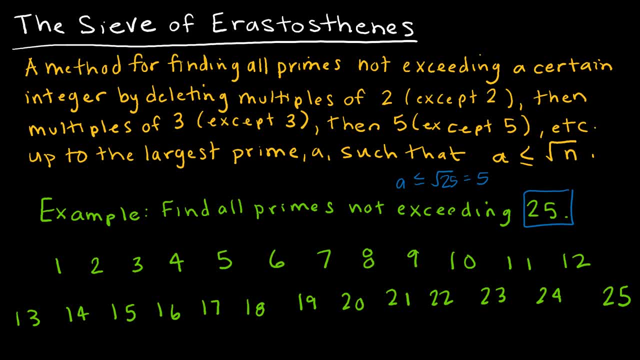 So I'm looking at all prime numbers, up to and including 5.. So how's this going to work? Well, first of all, I'm going to cross off 1, because obviously 1 is neither prime nor composite, So I shouldn't have even included that in the list. 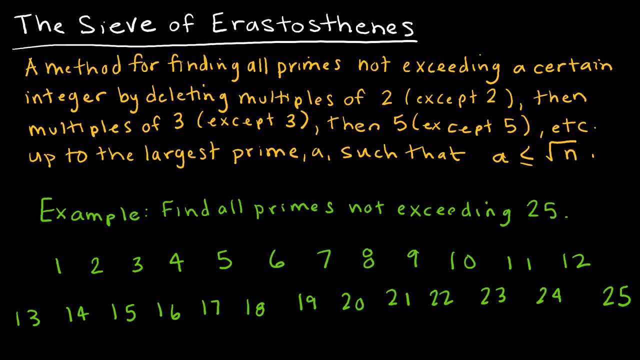 Then we're going to delete multiples of 3, because 3 is obviously a prime number, but we're not going to delete 3.. And then 5,, etc. through all of the largest primes, such that a is less than or equal to n. 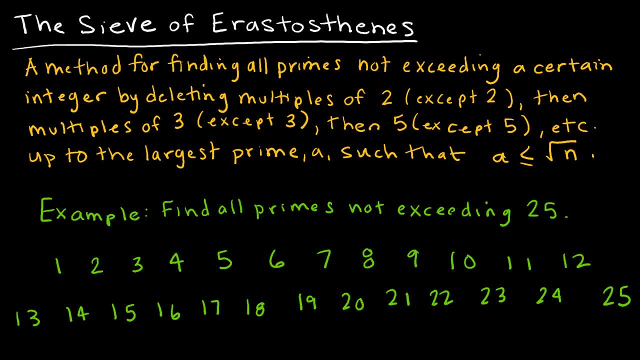 Sorry. a is less than or equal to the square root of n. So we're going to delete all of the largest primes, such that a is less than or equal to n. So I've given us a sort of a simple example. I'm using 25.. 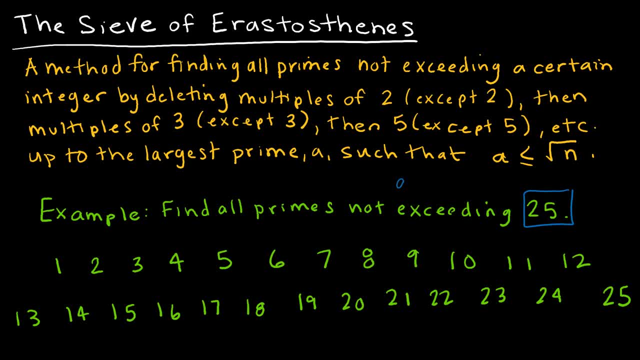 So I would take square root of 25.. So a is less than or equal to the square root of 25, which is 5.. So I'm looking at all prime numbers up to and including 5.. So how's this going to work? 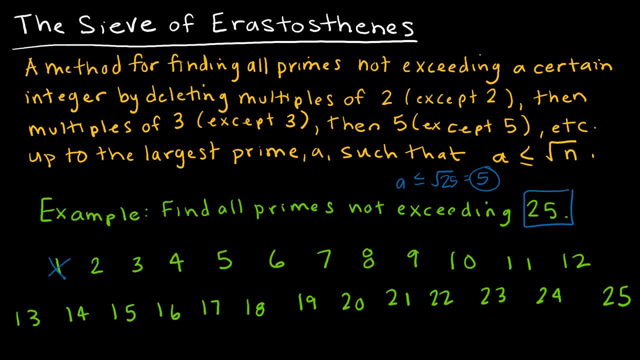 Well, first of all I'm going to cross off 1, because obviously 1 is neither prime nor composite, So I shouldn't have even included that in the list. But I can start then with 2.. I know 2 is prime, so I'm going to cross off all of the other multiples of 2.. 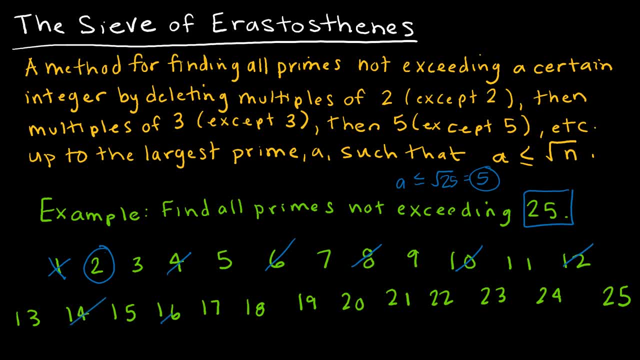 4,, 6,, 8,, 10,, 12,, 14,, 16,, 18,, 20,, 22, 24.. Notice, I'm up to 25, so that's where I stopped my list. Then I'm going to use the next prime, which is 3.. 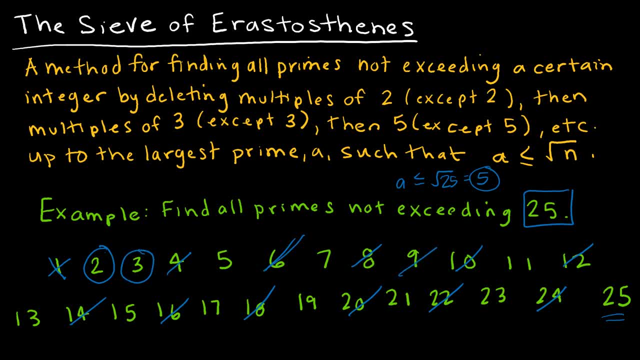 I'm not going to cross off 3,, but I'm going to cross off 6,, 9,, 12,, 15,, 18,, 21,, 24,, which are all the multiples of 2.. And then I'm going to go with 5.. 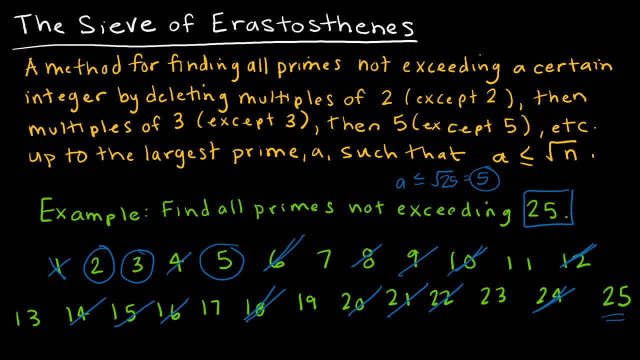 So 5 is a prime, and I'm going to cross off multiples of 5.. So 10,, 15,, 20,, 25.. This method then leaves only primes left over. So all of the primes that are less than or equal to 25 are 2,, 3,, 5,, 7,, 11,, 13,, 17,, 19, and 23.. 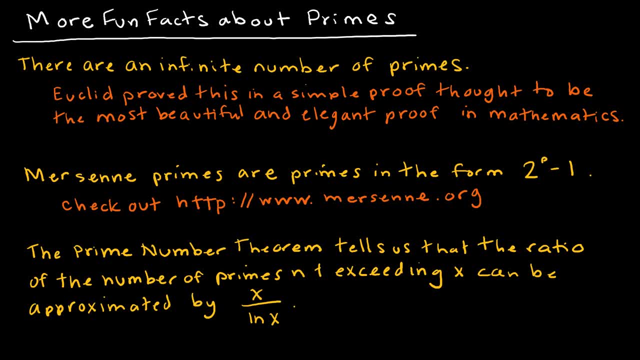 Here are some examples. Here are a few more fun facts about primes, and I'm not going to go over any of these little theorems with you. But one theorem says there are an infinite number of primes, and Euclid actually proved this. 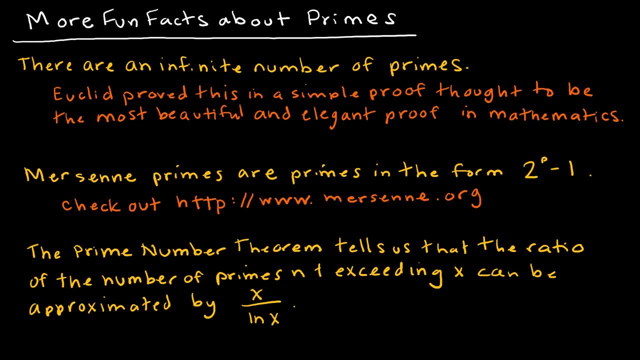 and thought it was the most beautiful and elegant proof in mathematics. So if you're up for Googling something, feel free to Google Mersenne. primes are primes in the form of 2 to the p minus 1.. And I have given you a website there if you want to learn a little bit more about that.